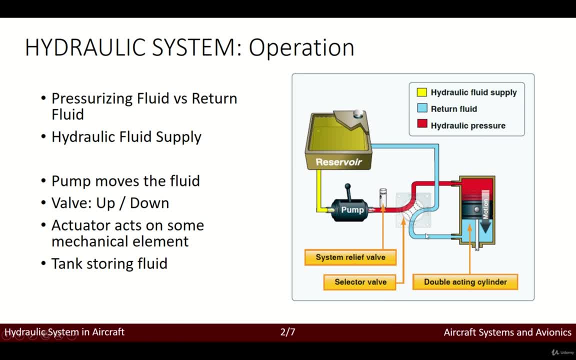 is a selector valve over here which will mainly indicate whether the fluid moves in this direction or it either moves on the other direction, okay. So again, what we have in general terms is a pressurizing fluid. okay, which is that pressure? you know that fluid which is? 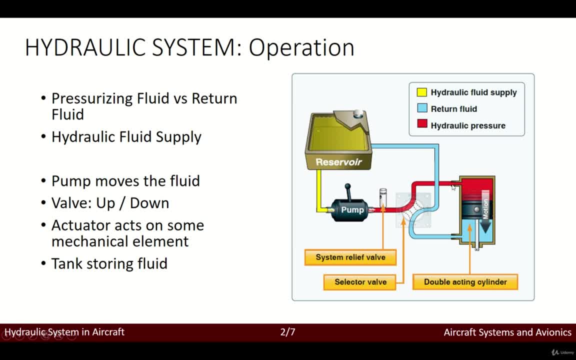 out an output of the pump, Then what we have is a return fluid in order to close the circuit. okay, with going back to the reservoir, And the main idea is that the output pump moves the fluid We have. the valve that might have you know it can have two positions. 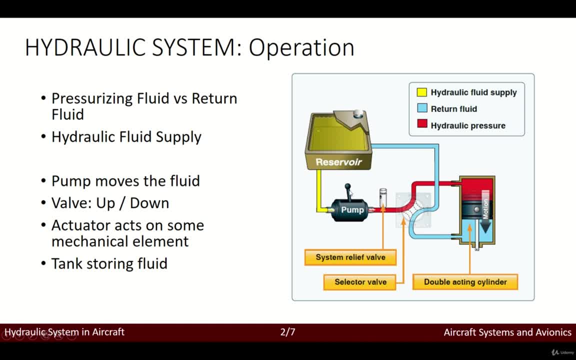 It can be described as up and down, okay, depending on which of the direction. you know, the direction of the fluid that we have, you know we happen to decide. Then what we have is the actuator that acts on some mechanical element And finally, the reservoir, which acts as tank. 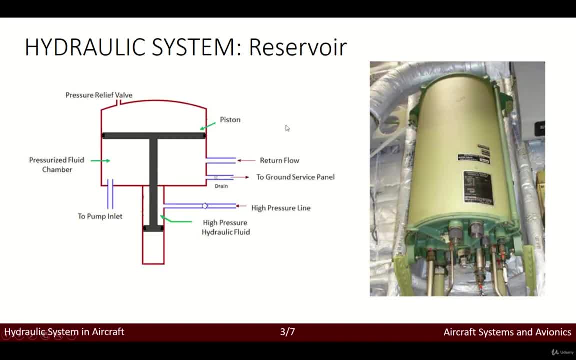 storing fluid right. So hydraulic fluid reservoirs are required by most aircraft systems in order to provide a ready source of fluid for the hydraulic pumps and also to contain, you know, a varying volume of fluid. This variance, okay, of fluid results from differential actuator. 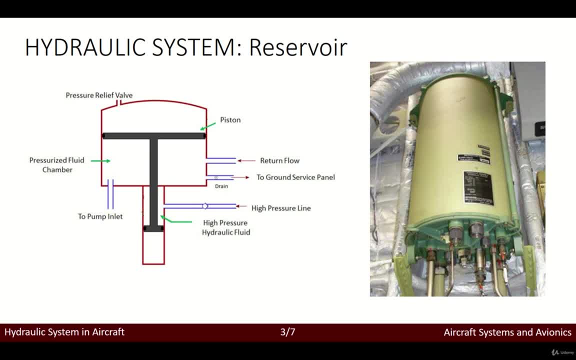 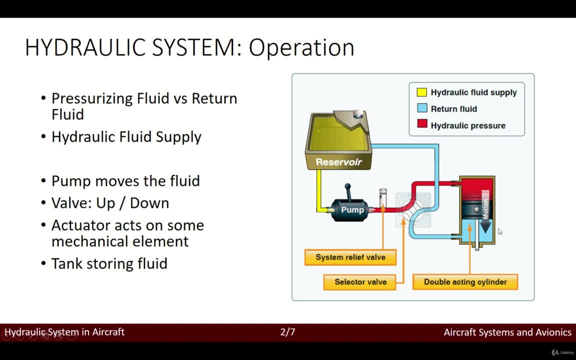 volume dependent upon whether the actuator is extended or retracted. Now, the main idea here is that if I go back, we have we might have different amounts of volume- okay- on one side and the other of the actuator due to the fact that 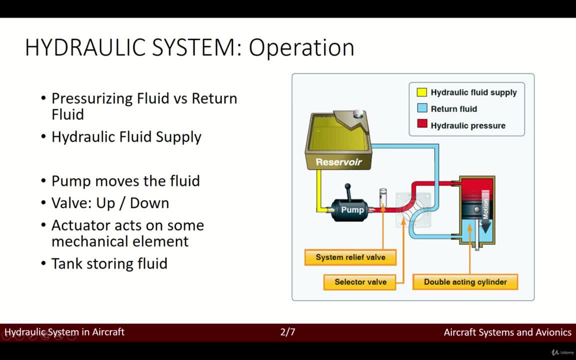 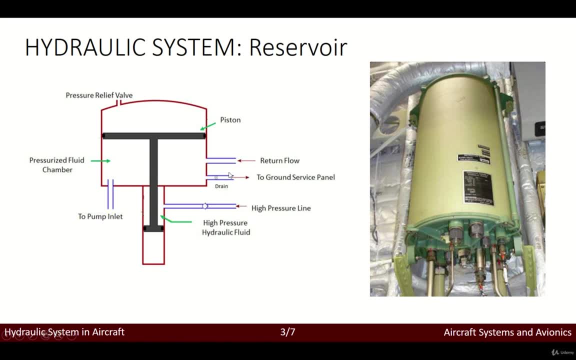 usually we will have, you know, a connector which is only on one side, okay, meaning that we will notice a bit of difference on the volume right. So the reservoir size is optimized so that only the amount of fluid needed for proper function is carried. okay In many installations. 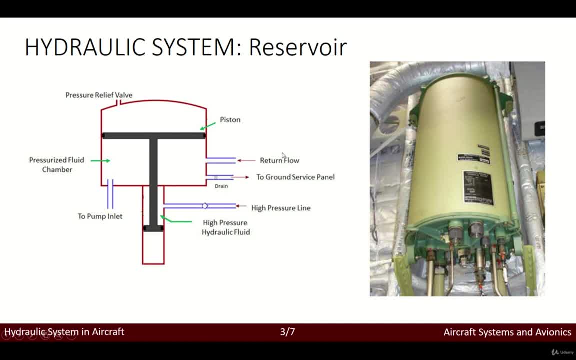 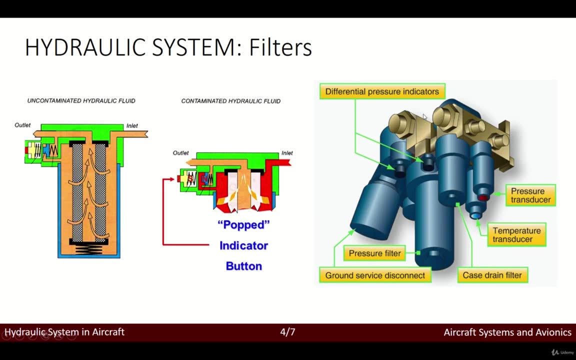 bleed air will be used in order to pressurize the reservoir, to help, you know, to help prevent hydraulic pump cavitation right or any instant instability due to low pressure. Okay, so, in addition to that, we also have filters, for instance, which, as you can imagine what we do. 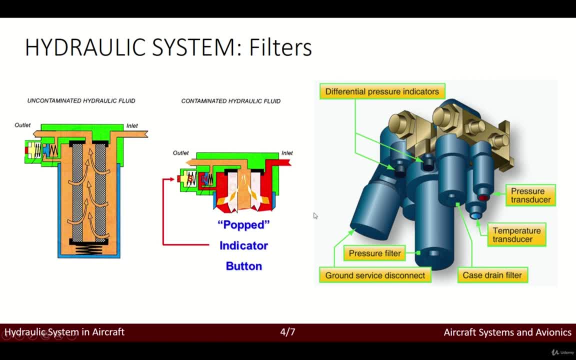 is eliminate any contaminated particles, you know contaminated fluid inside of the hydraulic system. okay, and basically, hydraulic fluid cleanliness is essential to proper system function. okay, Inline filters are incorporated into the hydraulic system in order to remove any contaminants from the fluid. The idea here is that we 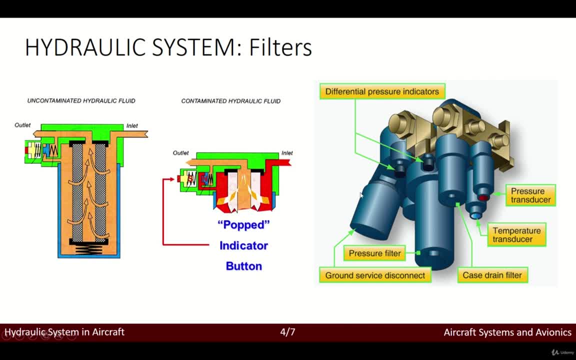 simply have, like a concentric cylindrical filter, okay, such as these ones, and what you see is we have an inlet which is on the outside of the cylindric cylinder, okay, and then it moves, you know, throughout a radial cylinder, which is a filter. it moves to the inside. 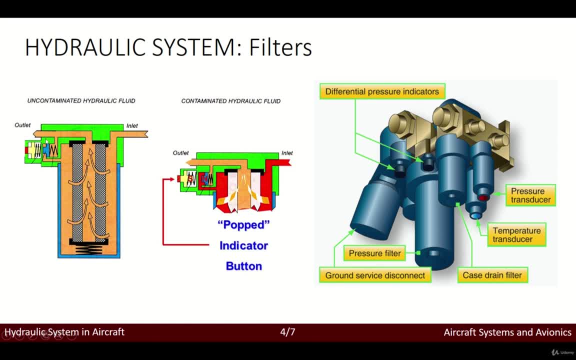 okay, and then just goes out, coming from the inlet to the outlet. This is the main idea of the filter. However, in the case of having a contaminated- you know liquid, okay fluid- what will happen is that this fluid will end up, you know, moving towards this direction. 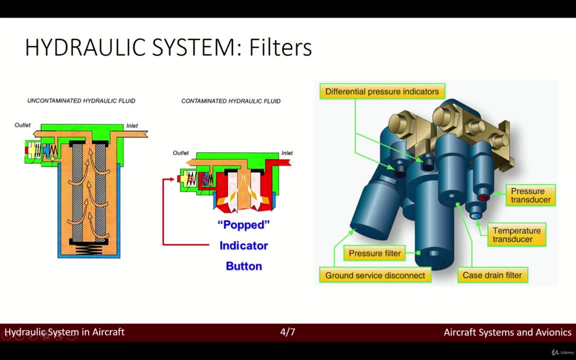 and if this happens, okay, because of additional particles, then usually due to magnets or using several techniques, we will actually be able to have this piece moving over here. okay, in fact, it's moving the other way. So, basically, what will happen is that we will get a notificator, okay. 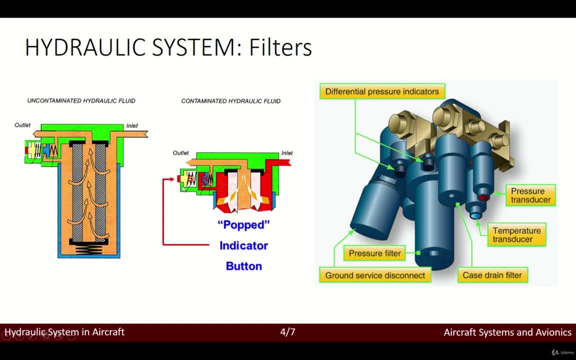 some kind of button on the outside popping out indicating, right, that the system you know that the hydraulic system has some contaminants on it. Then it is, you know, a question of maintenance to make sure that all of this actually works and the hydraulic system you know has no contaminants on it. okay, This is. 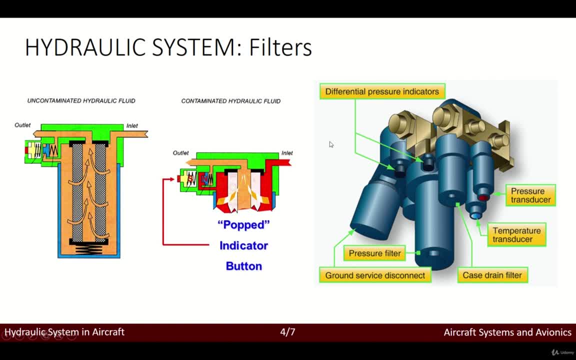 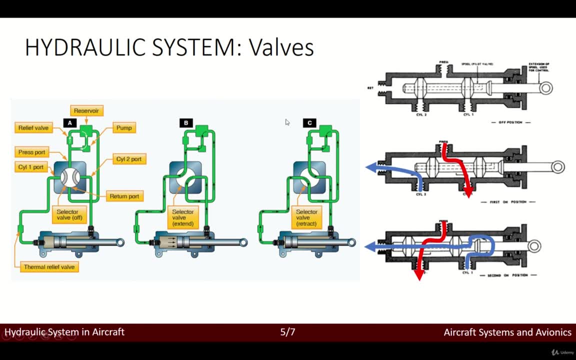 actually a crucial part of the hydraulic system. You have to make sure in all cases that the filters are operating normally. This is the idea of the valve control valves. okay, Hydraulic motors and actuators have an associated control valve which is positioned in response to a manual or automated system selection. 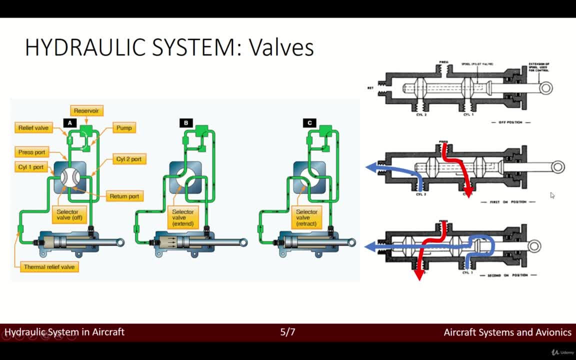 okay, such as a moving, you know, such as moving the flap lever, for instance. So basically, we have a way, a manual, automatic way to control this. okay, And the main idea of a hydraulic system, you know, sorry, of the valve, as you can imagine, is just 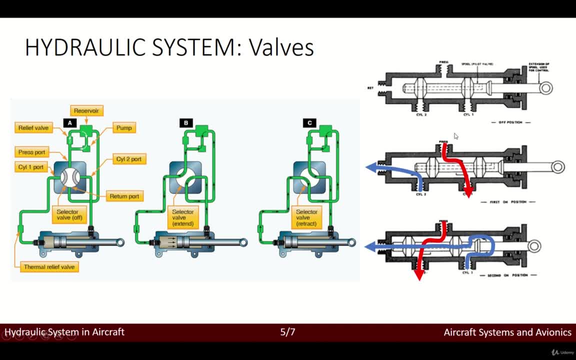 this is some- I'm not sure the name of this kind of system, but basically what you will have as a valve is some kind of piece which is moving in some way or another and providing one direction or other to the fluid. okay, As you can see on the red line over here the you know the fluid is moving on. 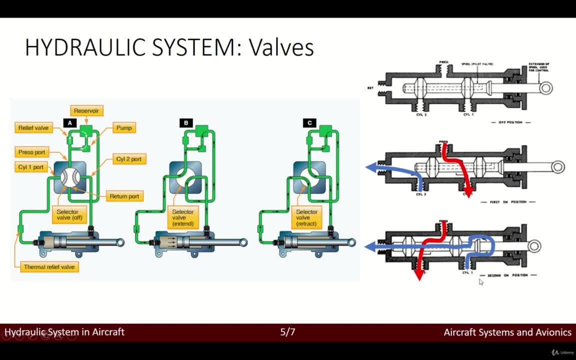 this direction, towards this position number one over here, but instead- okay in the first case, but instead on the second case it's going to the other direction And because we have these interior tube over here, we're actually able to provide also the you know, to make sure that the 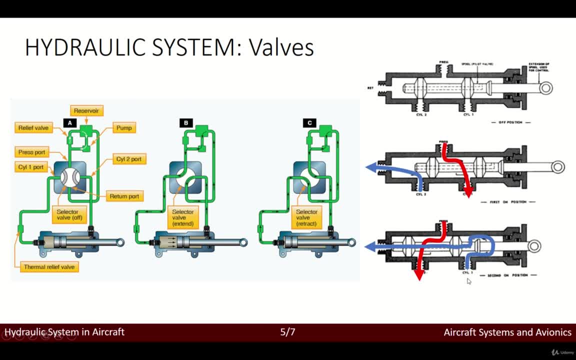 from number two it can go outside, like this, but also from number one it can go through the tube, through this inside tube- okay, to the outside also. So basically, again, what you need to provide is a means to make sure that you can change the direction. considering an input. 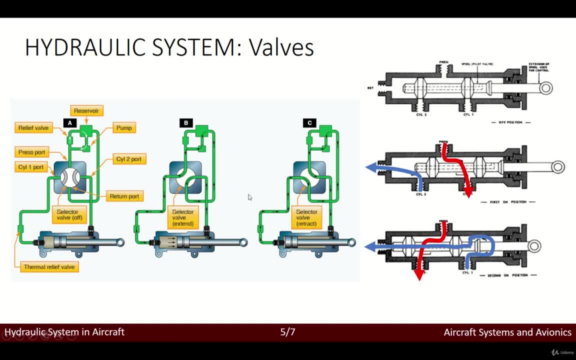 okay, considering the position of this flap, for instance. I think there's nothing more to to add here, just a basic like notion. okay of this is a controlled valve, meaning that we can actually control both sides, right. however, we have, you know, plenty of valves, types of valves. 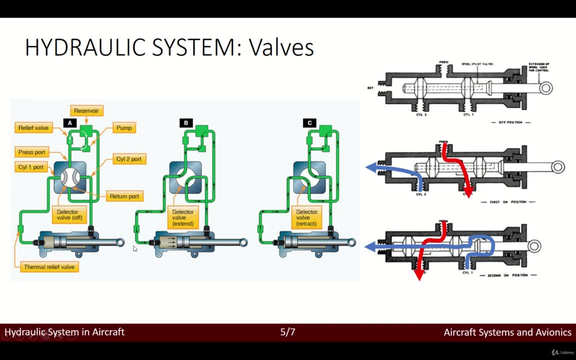 There's so many types of valves, depending on the type of operation, that we need to use. okay, Maybe, instead of having two tubes, okay, going to one direction and the other direction. I'm kind of balancing this piston over here. What we have is only one and you know we could have on another side. 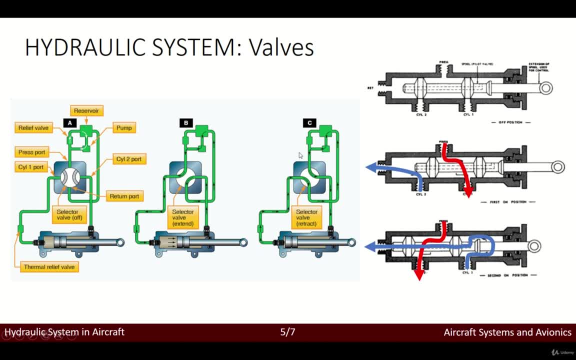 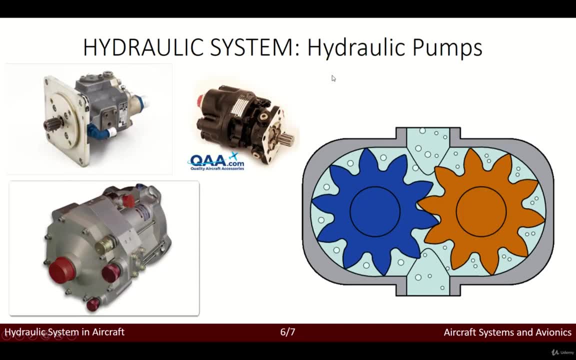 simply have a spring, for instance. so it really depends on the type of of the system, okay, but this is the most generic case, right? and finally, what we get is the hydraulic pumps. pumps, okay, so pumps are frequently mounted on the engine accessory gearbox. it might depend and the way. 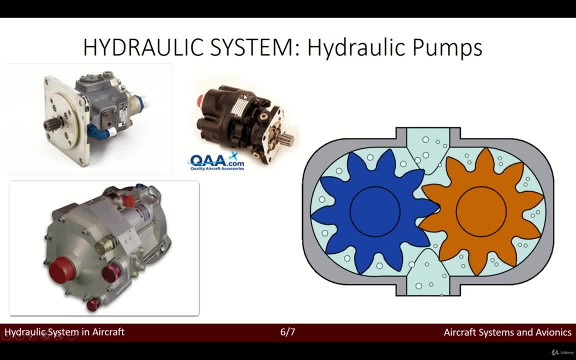 that we actually actuate these hydraulic pumps can be, you know, by many means again, so maybe electric. both ac and dc motors are utilized to power hydraulic pumps, usually with three-phase ac motors being the most common. okay, we also have nomadic, which would you know be using the bleed. 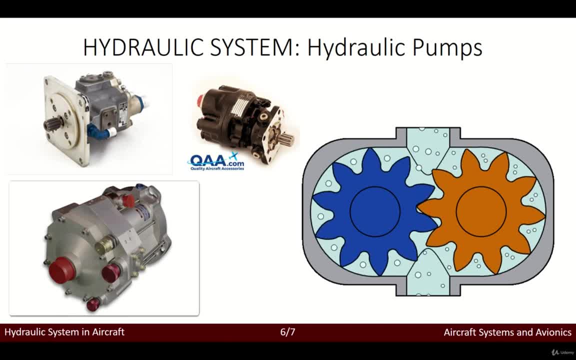 air powered motors, which is also utilized on some aircraft to drive hydraulic pumps, and you know there's several more types. but the main idea here is that we basically have an outside element which we have to control, okay, which we have to move by using electric or pressurized or, you know, nomadic systems. that depends, but the 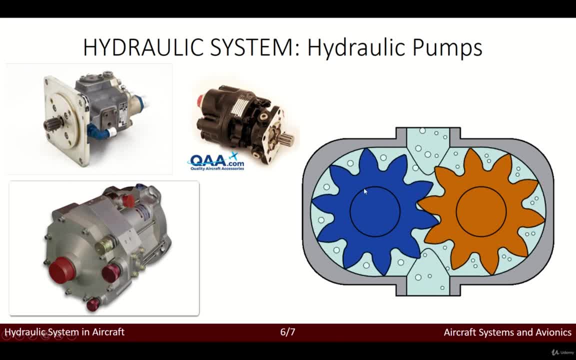 main idea here is that we actually need to move that, and once we start moving that, we start moving this. you know this blue rotating elements over here. okay, what we have is that the fluid will start moving from one side to the other at a certain pressure. okay, so this is what we are. 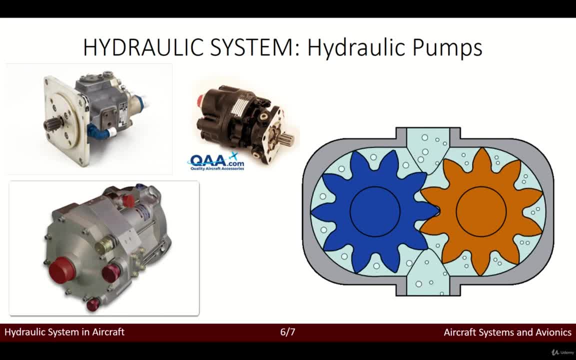 generating by using the hydraulic pump. okay, so yeah, this would be a bit of the schematic of what the hydraulic system looks like. this is for all hydraulic systems. in the case of the aircraft, you can see it in in several items, such as the landing gear and the flaps. maybe they are the 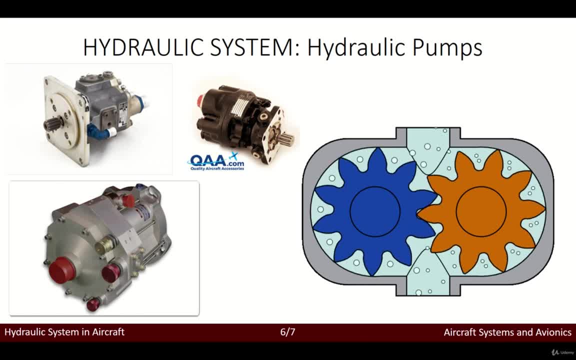 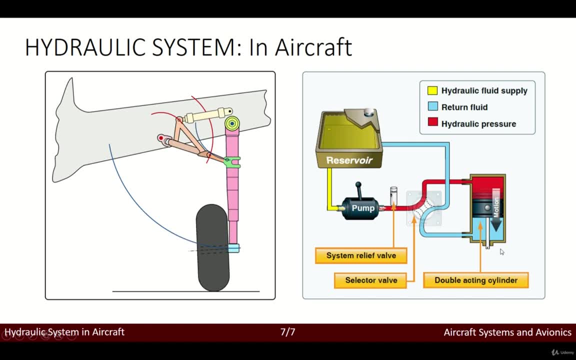 most common, but also in the case of our ailerons and control surfaces on the tail, okay, and this is a bit of the schematic again, or in the case in the aircraft. so, as we've seen, this would be the actuator, okay, having a, you know, a control valve, as we mentioned before, allowing for the fluid to move. 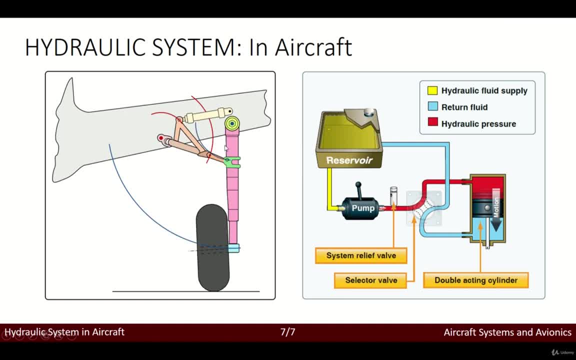 in the in the two directions right, and here we have the example of an actuator acting on the landing gear and retracting the landing gear. okay, so again because of you know, by moving this element over here, what we actually are capable of producing a mechanical work on the. 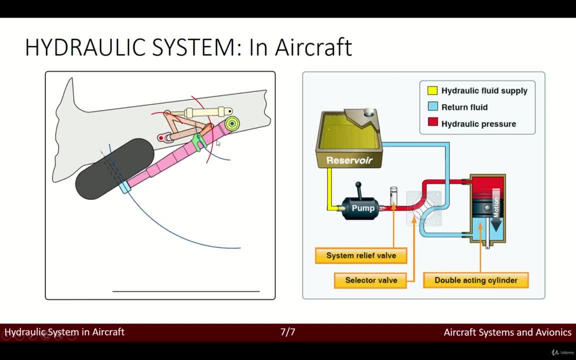 landing gear, okay, making sure you know the piston. by moving the piston, we can make sure that we're retract, or I'm not sure what the word is for the contrary, but the idea is either retract or get the landing gear out. okay, so this is what you will be capable of doing by using the hydraulic system. okay, so now we can go to the next class.